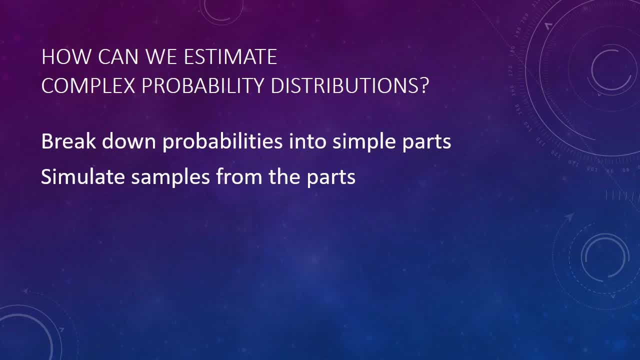 Anyway, we use the computer's coin flips to represent outcomes from the simple probability distributions. Next, we combine the simple outcomes from each of the simple parts into complex outcomes from the complex distribution we're interested in. Finally, we use counts of the simulated outcomes as an estimate of our complex probability distribution. 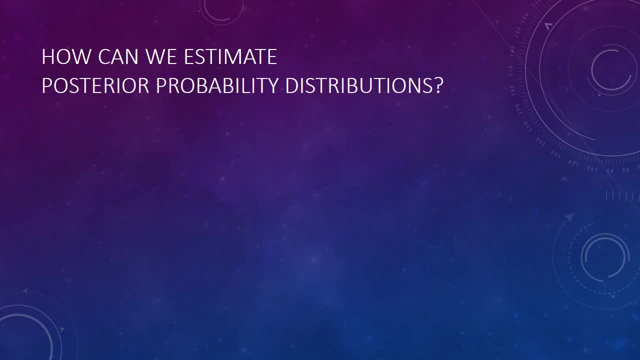 To be a little more specific. if the complex probability distribution we're interested in is the posterior, we can break down the posterior into simple pieces using Bayes' theorem. The posterior is simply the likelihood times the prior divided by the marginal probability of the data. 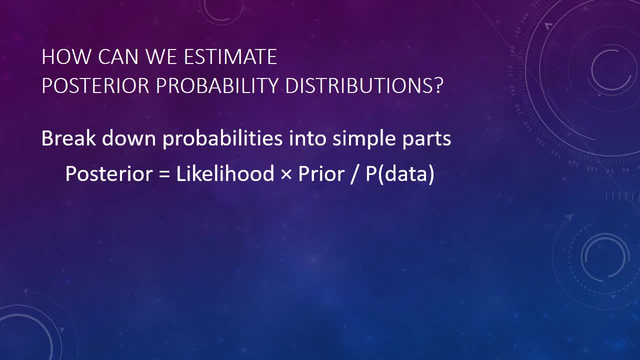 Each of these simple parts- the likelihood and the prior- is fairly easy to simulate. Next, we need a way to combine the outcomes from each part- the likelihood and the prior- into complex outcomes. For this we'll use a technique called Markov Chain- Monte Carlo. 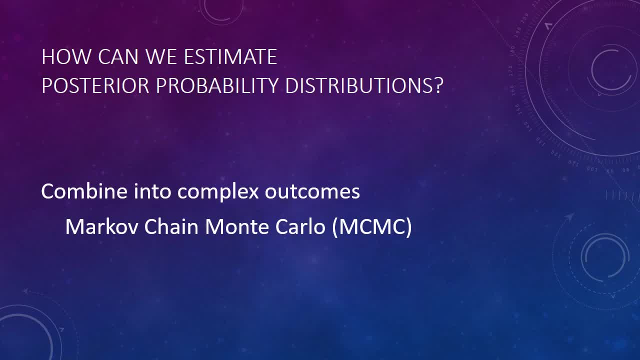 Or MCMC for short. The gory details of how MCMC works are beyond the scope of this class, But let's see if we can understand the gist behind the madness, And for that a story. Jack and Jill went up the hill every single day. 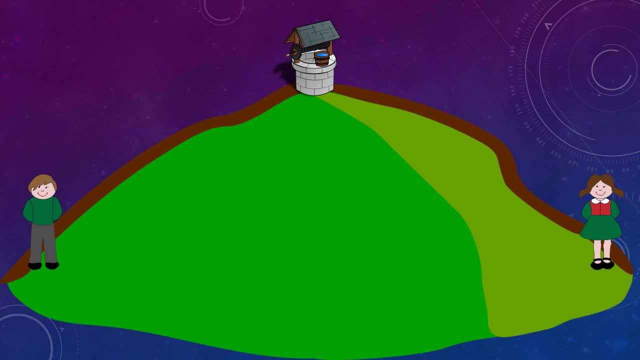 Oh Jack, said Jill, I'm tired of going up this hill, It's so boring. Can't we make fetching water any more interesting? I know, let's play a game, said Jack, Instead of just going straight up the hill. 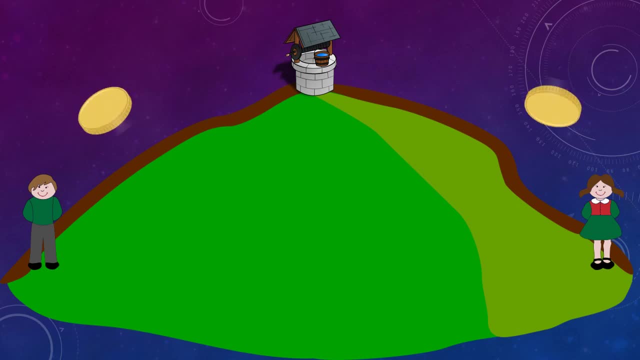 let's flip coins: Each time we get a head, we'll take a step up the hill, And each time we get a tail, we'll take a step down the hill. Jack said, Jill, we'll be taking one step back for every step forward, on average. 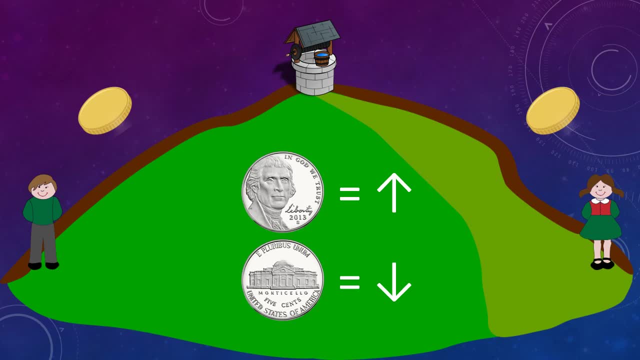 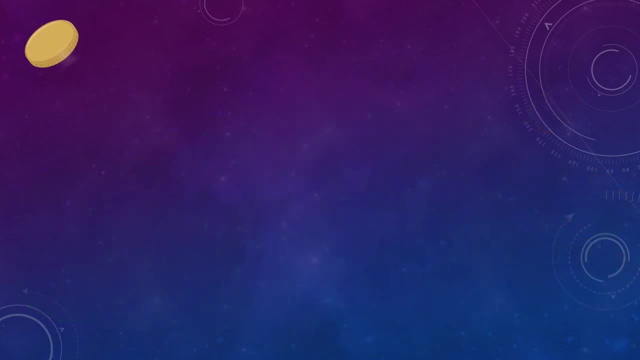 And we'll never make it up the hill to get water in time for Ma to make soup for supper tonight. Okay fine, said Jack a little indignant. Let's make it a little more interesting. We'll still flip a coin to see whether we go up or down. 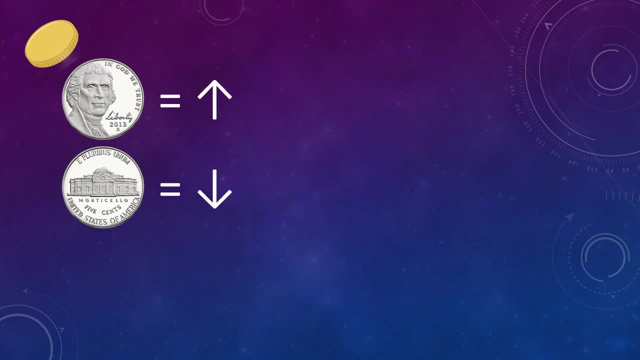 But if the coin comes up tail, before taking a step down the hill we'll flip the coin a second time. If it comes up tails again, then we'll go ahead and take that step down the hill, But if it comes up head the second time, 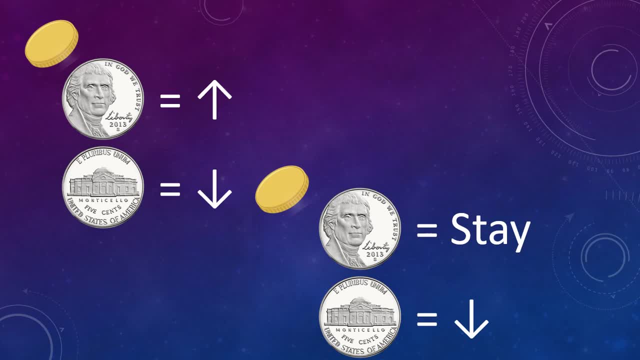 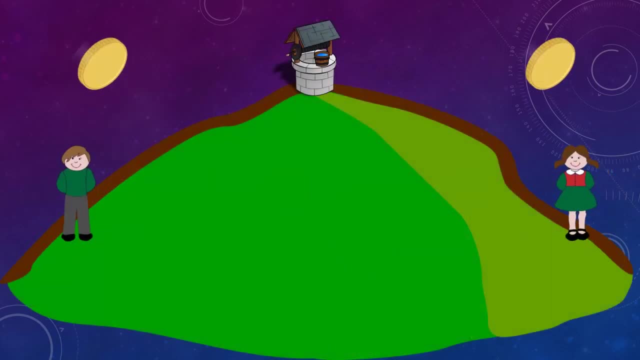 we'll just stay put. That way we're more likely to make progress up the hill, but we still have a chance of going backwards. just to make things interesting, Let's give it a try, said Jill, And they started flipping coins and taking steps forward and back on the hill. 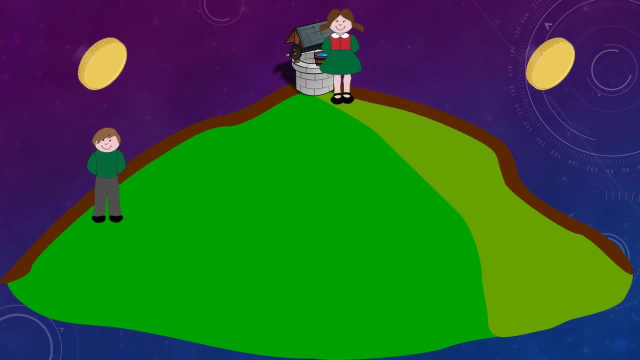 They must have looked pretty silly to any passersby walking up and down the hill Like drunks, But they had a splendid time at it And because they set up the game so that they were more likely to go up the hill than down. 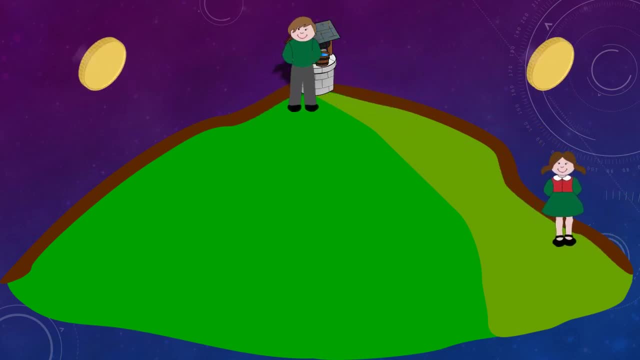 they ended up spending more time toward the top of the hill, where the well was, than at the base of the hill, which was far less interesting for drawing water for supper. The story with Jack and Jill illustrates Markov Chain, Monte Carlo, which, as the name suggests, 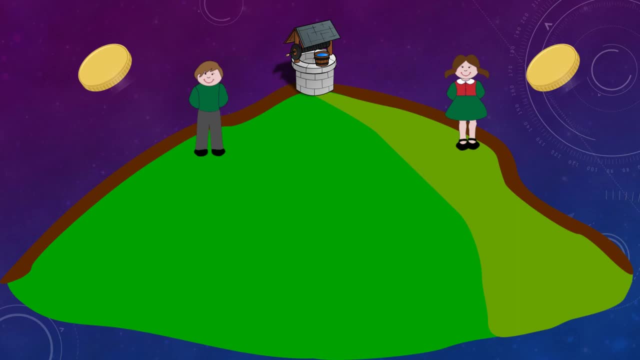 is a chain of steps through perimeter space, that is, through the space of all the possible models. The steps from one possible model to the next are all random, but the jumps are set up in a way that you spend more time with models that are more plausible. 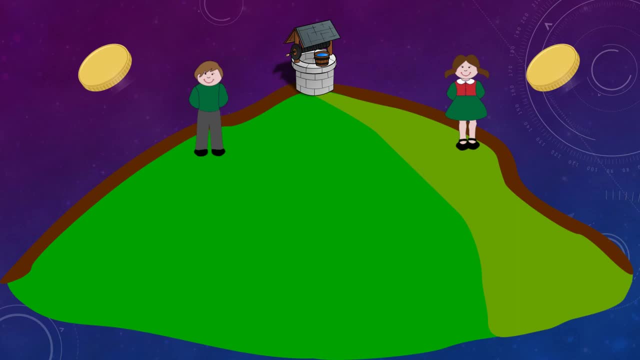 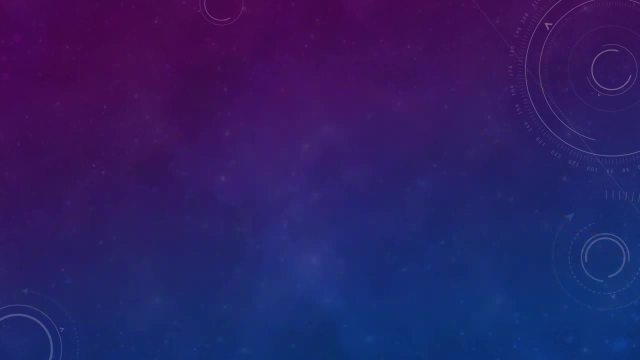 and less time with models that are less plausible. Jack's game is very similar to a common algorithm for MCMC called the Metropolis-Hastings algorithm. In this algorithm, you first flip a coin to determine whether to go up or down in the perimeter space. 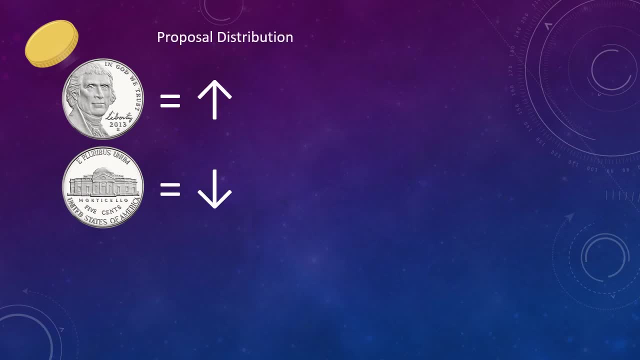 This is called the proposal distribution, because it proposes what step you should take next. If the proposed model is more plausible than your current model, you take the step, But if the proposed model is less plausible than your current model, you flip a second coin. 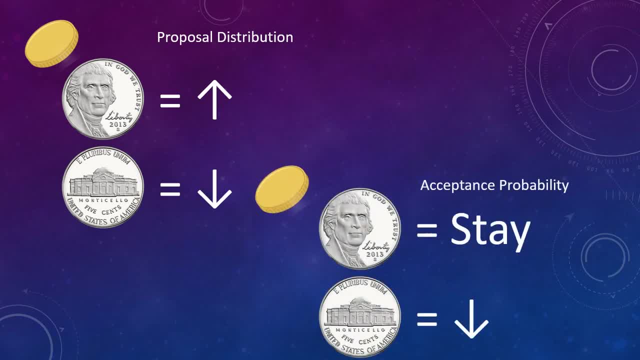 to determine whether to actually go through with the proposed step. This is called the acceptance probability In the Metropolis-Hastings algorithm. you accept a less favorable step in direct proportion to how unfavorable it is. You accept slightly unfavorable jumps much of the time. 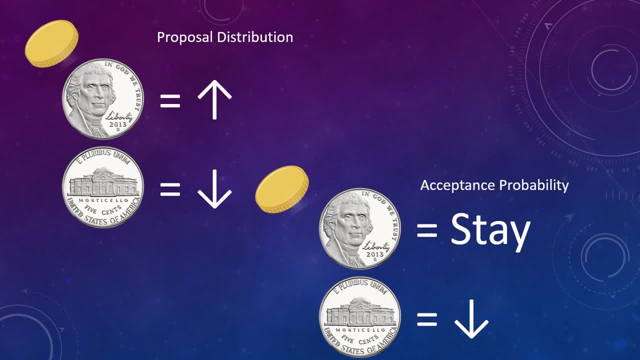 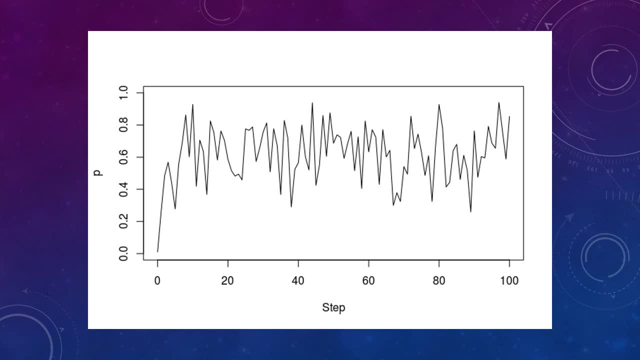 but you accept very unfavorable jumps only. The result of all this jumping is a record of all the places you've visited along the chain, like a video of how far up the hill Jack and Jill were at each point in time. Like Jack and Jill,